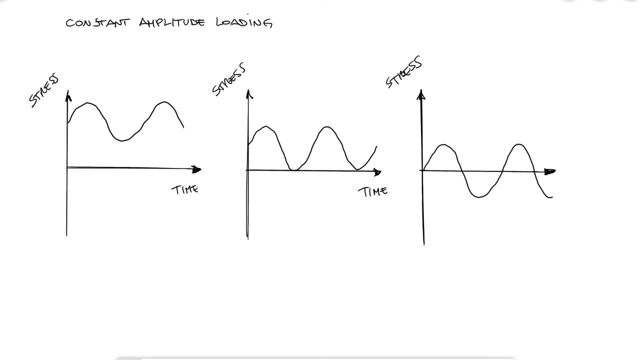 of terms that we will be using regularly. The mean stress is written as sigma m, and it's the average between the minimum and the maximum stress, and the alternating stress or stress amplitude is, of course, the amplitude or the distance between the minimum and the maximum. 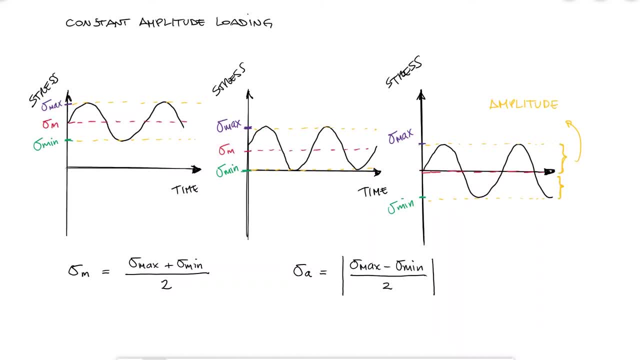 stress over 2.. We call fluctuating stresses of constant amplitude a completely reversed stress, when the mean stress is zero, since the minimum stress value is just a negative value of the maximum stress. These completely reversed stresses are pretty common and will be useful. 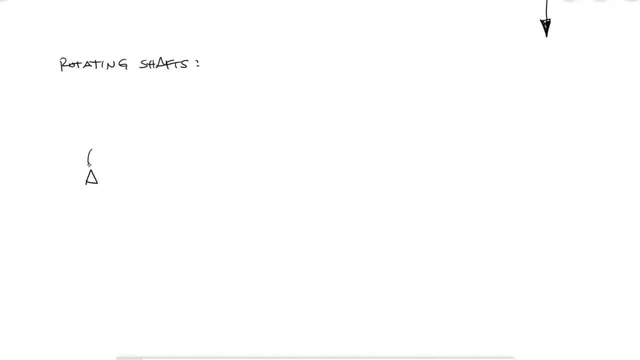 for many of the applications we will study in this course, like, for example, shaft design where bending stresses vary from negative to positive sigma continuously while rotating. This notion is exactly what we use to experimentally measure this fatigue strength property that I mentioned before A bending machine is used on. 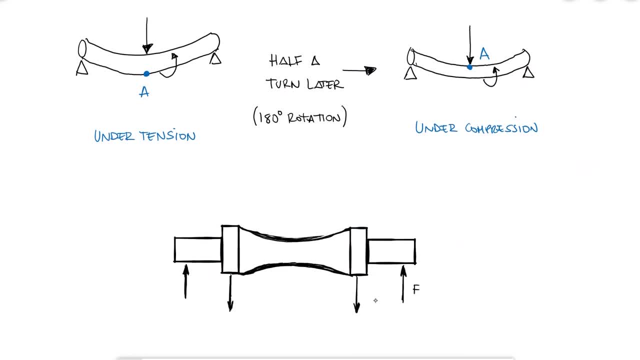 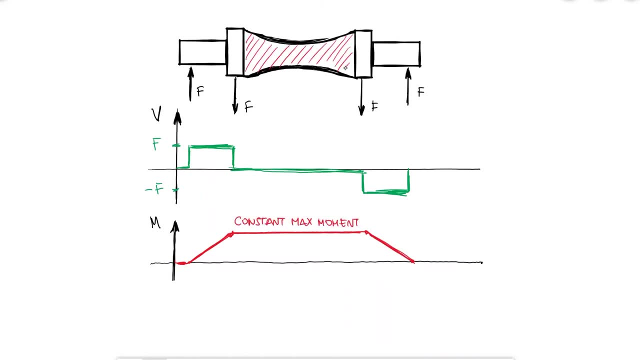 a specimen to cause a known bending stress that is highest at the center. If we look at a quick transverse shear and bending moment diagram, we see that the moment is constant throughout the middle section And because the cross-section area is smallest at the center, the maximum bending stress will occur exactly there. 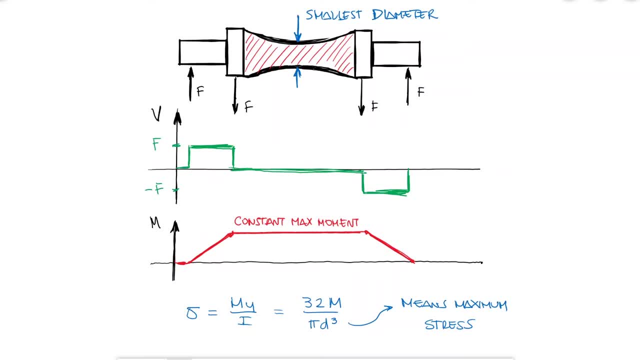 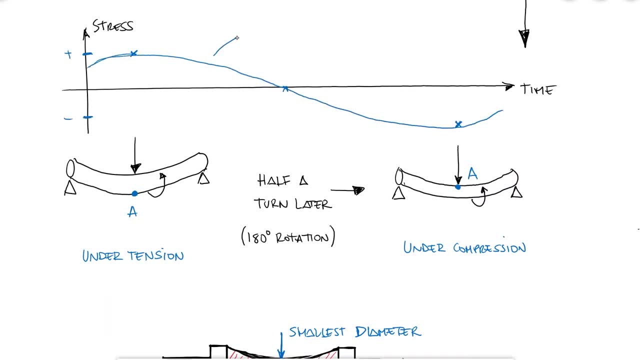 Since the specimen is constantly rotating, a specific point on the surface of the rod will go from a positive normal stress tension to a negative normal stress compression of the same stress value and, of course, everything in between, If identical specimens are tested using distinct stress values until they break. 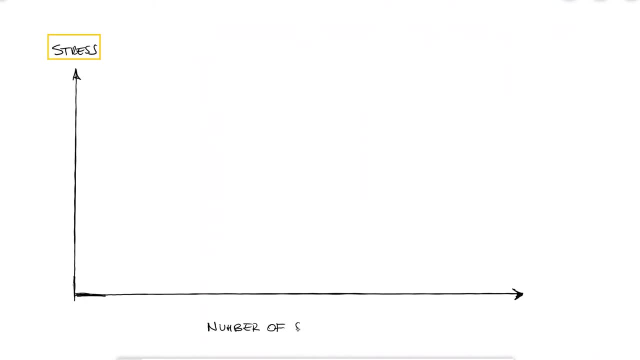 we would see that the specimens that are subjected to completely reverse stresses of low magnitudes break after many cycles, while specimens subjected to completely reverse stresses of higher magnitudes break after fewer cycles. If we do this for several values of alternating stress, we develop a plot that we call the SN. 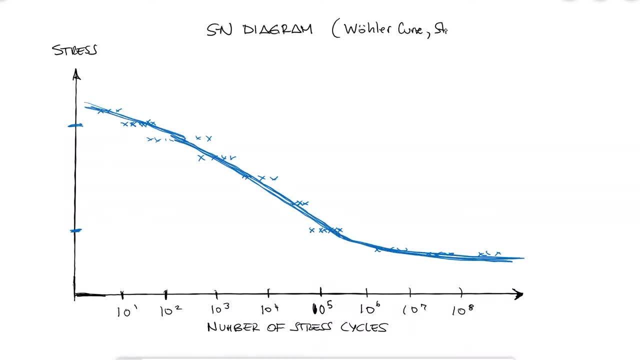 diagram, sometimes, but not often, called Volea curve or stress-life diagram, where the y-axis, which records the stress that was used and ultimately made the sample fail for a specific number of cycles, is called the fatigue strength. Failure with less than. 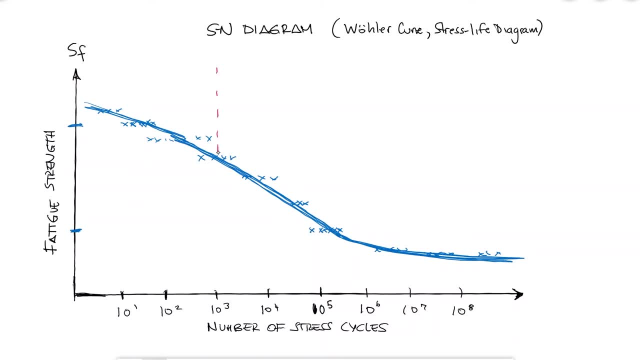 1% of the stress value is called the fatigue strength. Failure with less than 1% of the stress value is called the fatigue strength. Failure with over 1000 cycles is usually classified as low cycle fatigue and failure with over 1000 cycles as high cycle fatigue For some materials that never fail for stress. 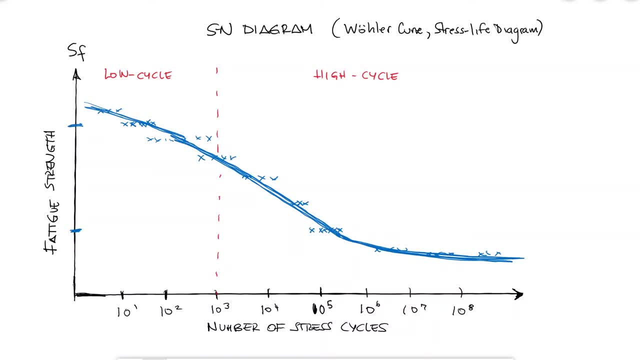 levels below a certain threshold, and by never we usually mean 100 million to 1 billion cycles, as it would be impossible to test for infinite cycles. the fatigue strength value for that threshold is called the endurance limit. Stress values below the endurance limit will. 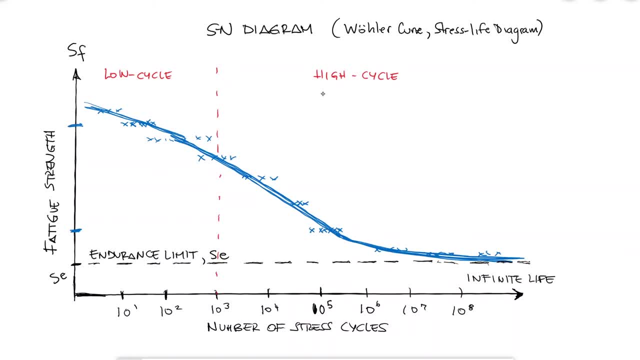 guarantee that the part will have infinite life. Depending on the material, the value for this curve will obviously change, and actually for some materials there is no such thing as an endurance limit, like aluminum alloys, for example. However, the overall behavior or shape, 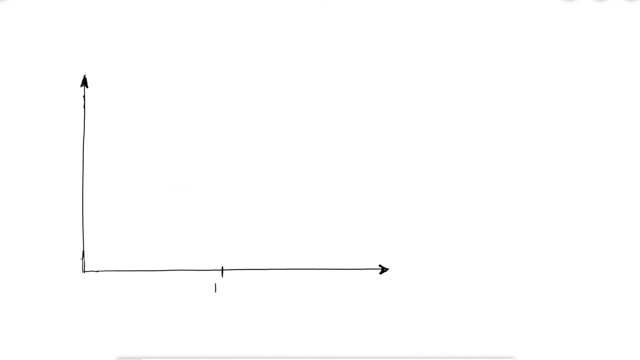 of this plot is similar And for this reason, for preliminary and prototype design, a simple, idealized yet conservative version of the SN diagram is very helpful. The low cycle region, for 1000 cycles or fewer, is represented by a line that has a gentle slope and that runs between the 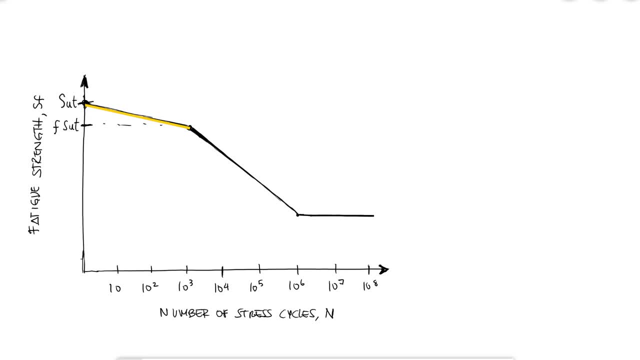 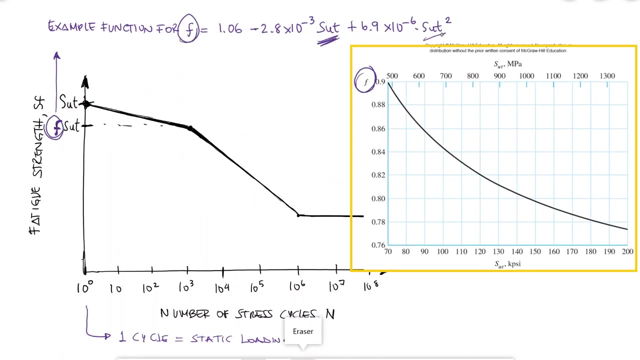 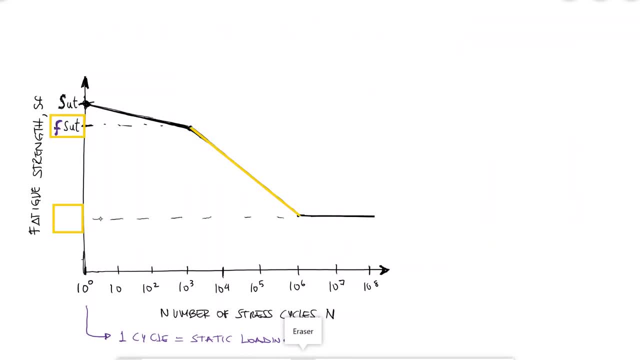 before infinite life goes from Fsut to the endurance limit. The endurance limit can be estimated for steels as half the ultimate strength for SUTs below 200 ksi, or the equivalent 1400 MPa, and 100 ksi or 700 MPa for any material that. 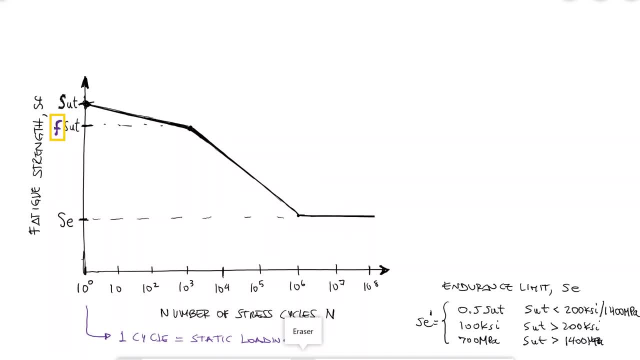 has a higher ultimate strength. Relationships to find both F coefficients and endurance limits for different materials can be found online or in textbooks and engineering handbooks. One of the most important capabilities from this idealized and again conservative diagram is being able to relate fatigue strength to number of cycles, especially for the high cycle region. 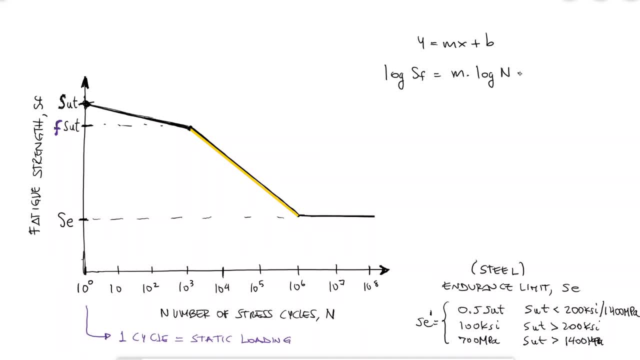 Since this region is represented as a straight line in a log-log scale, we know that Sf is equal to a times n to the b, just like we did on our previous video of crack propagation Link in the description below. If the fatigue strength Sf, 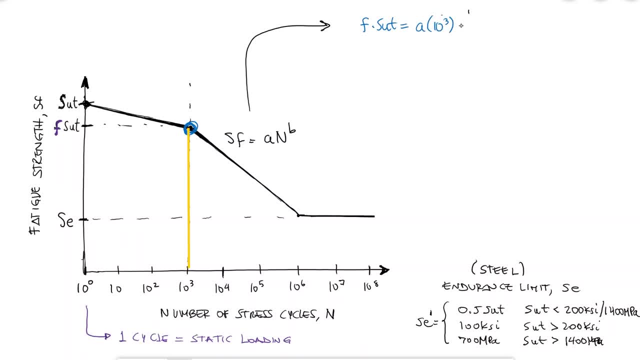 is equal to Fsut for n equal to 10 cubed, and Sf is equal to Se for n equal to 10. to the sixth, we obtain two equations with two variables: a and b. If we divide the equations, we find an expression for b and if 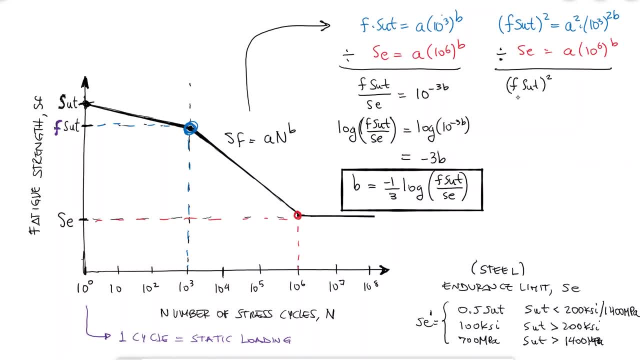 we square the first equation and divide again, we find an expression for a. If we're looking to find how many cycles a part would last for a specific, completely reversed stress, we can assume that the part will fail when that stress sigma ar, is equal to or exceeds the fatigue strength Sf and. 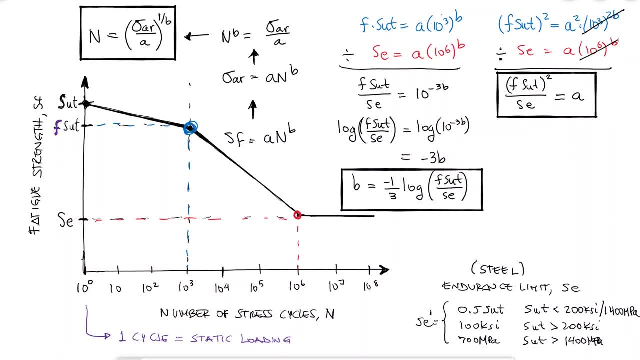 solve for n. The S-n diagram only applies to completely reversed stresses, but in future videos we will see how to transform any fluctuating stress to make use of the S-n diagrams. Let's take a look at a quick example. A rotating beam made out of a 10-20 steel has an ultimate. 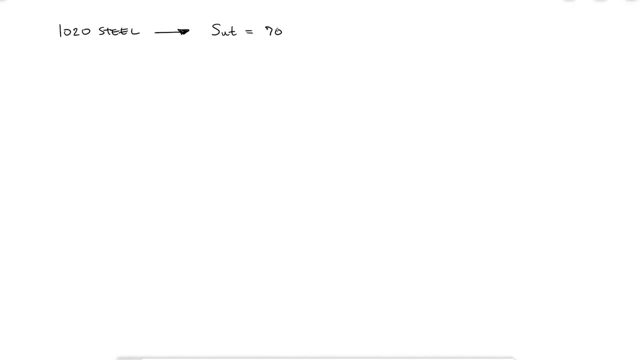 strength of 70 ksi. If the specimen is subjected to a completely reversed stress of 45 ksi, what would the factor of safety be for 10,000 cycles and separately, how many cycles would it endure before failure? The first thing I know is that the estimated endurance limit is 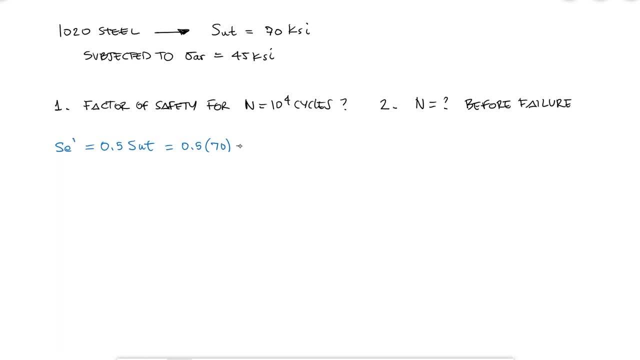 0.5 the ultimate strength. since the ultimate strength is below 200 ksi, The F-factor for a steel with an ultimate strength of 70 ksi would be 0.9.. By using the expressions that we just derived, I find that the coefficient a is equal to 113.4 ksi and the b-coefficient is equal to. 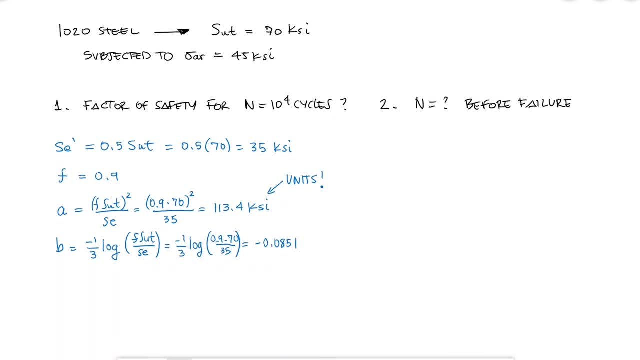 minus 0.0851.. Therefore, for 10,000 cycles, the fatigue strength would be equal to 51.8.. If the beam is being subjected to a completely reversed stress of 45 ksi and the fatigue strength is 51.8,, then the F-factor of safety is 1.15.. 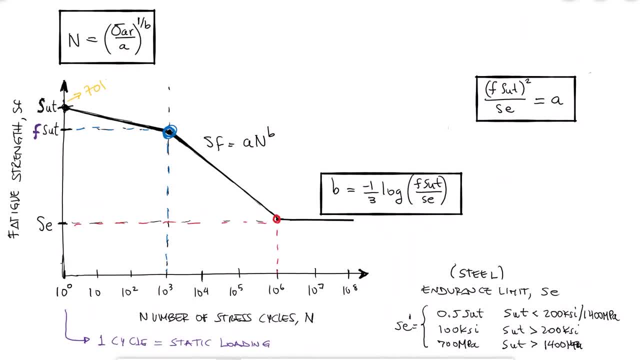 If I take a look at the S-n diagram to see what I just did, I would see that for 10,000 cycles the fatigue strength is 51.8, but I'm only subjecting the specimen to a stress of 45.. 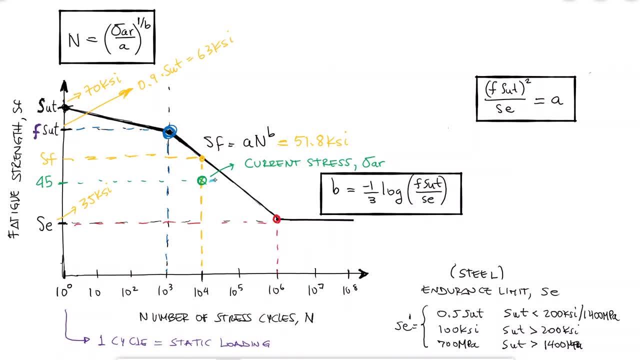 Now to answer the second question. I need to use the same equation and solve for n, knowing that if the part is going to be added to the beam, that the beam will be subject to a completely reversed stress of 42 ksi per 10,000 cycles.